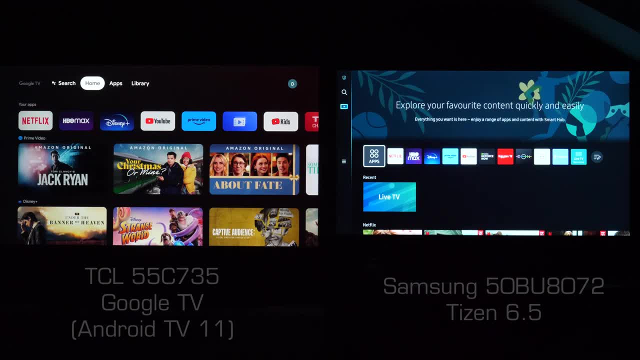 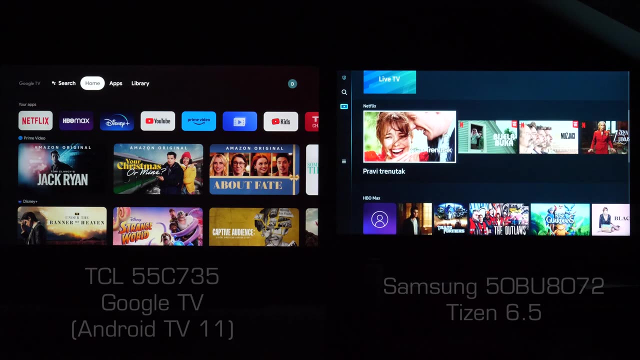 Explore your favorite content quickly and easily. There is a line with apps which you can arrange as you like. Below is recent input that will preview content from that input and then recommended content. You can also view the content from different streaming services, so similar to Google TV. 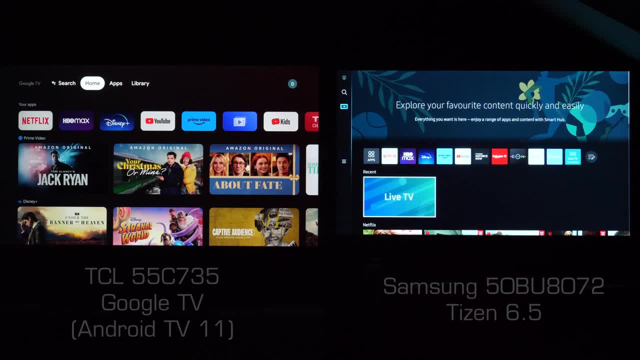 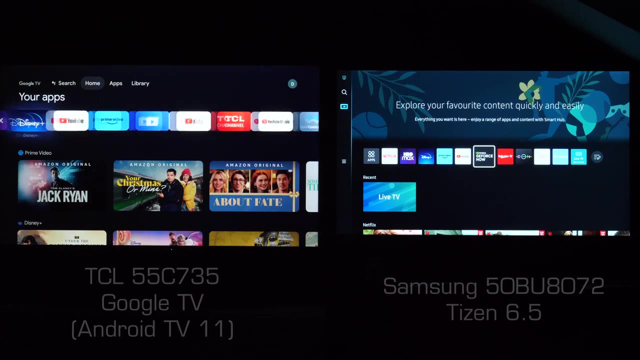 At the end there is this arrow. If we press it, we are back to the top In terms of customization of home menu. what you can do is rearrange your apps here and on Tizen. The easiest way is to simply long press OK button on the app you want to move and then choose from. 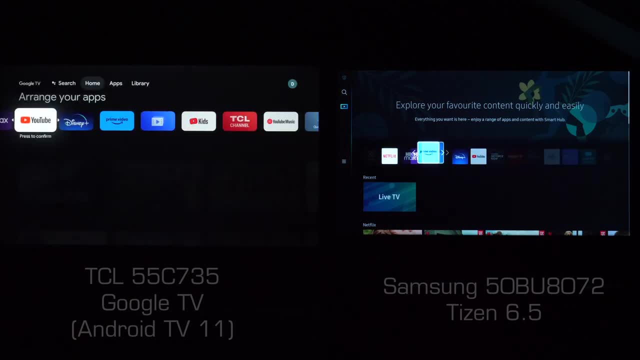 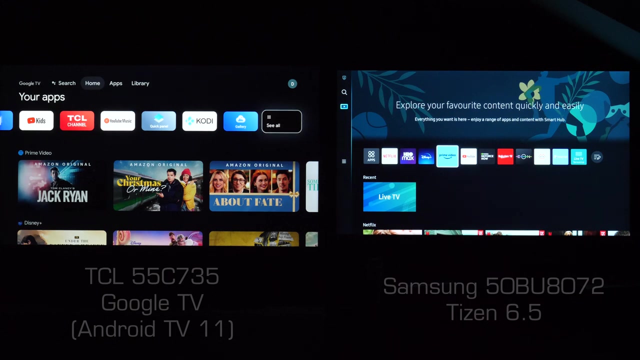 this menu. Let's go with move and then you move it to the position you want. So if you are often watching YouTube, you can put it on the first position, and so on. You can also go all the way to the end of the line. press see all on Google TV and you will see. 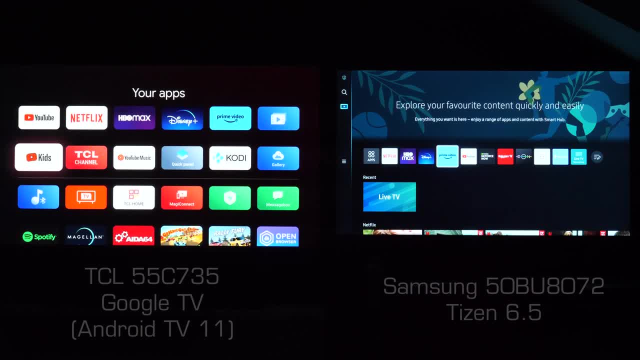 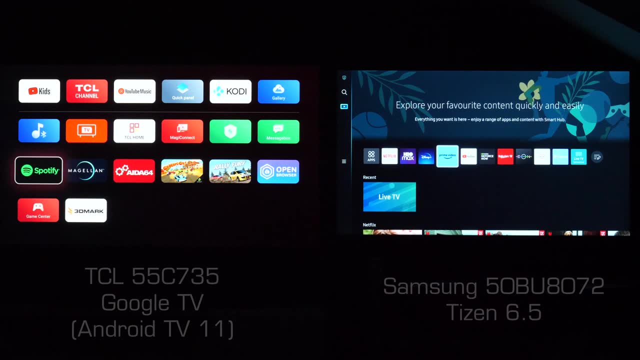 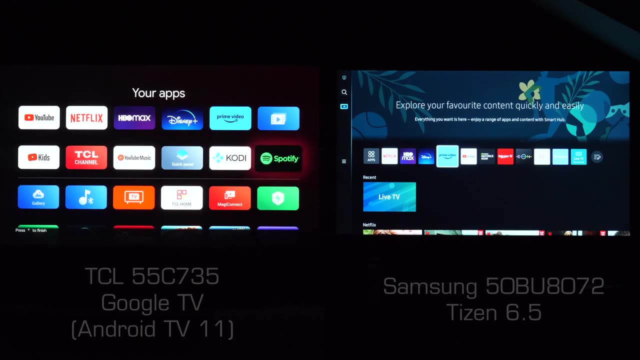 all the apps which are installed and apps which are above the line will appear on the home menu. So if you want to show some other app like Spotify, let's long press it, select move. move it to the top, press OK. When we go back to the home menu, you see Spotify here. 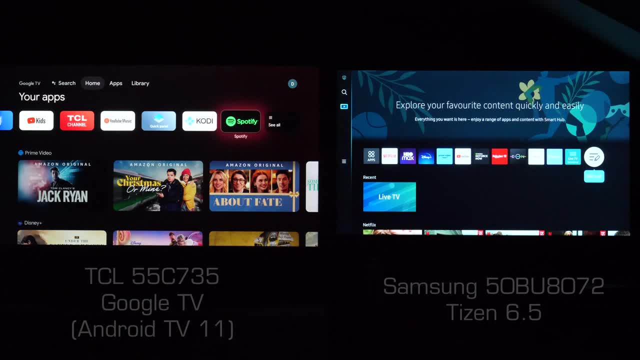 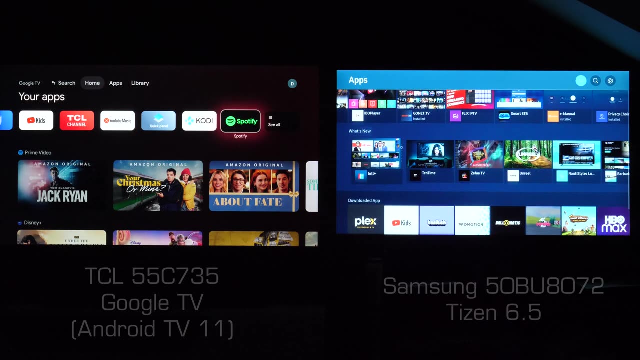 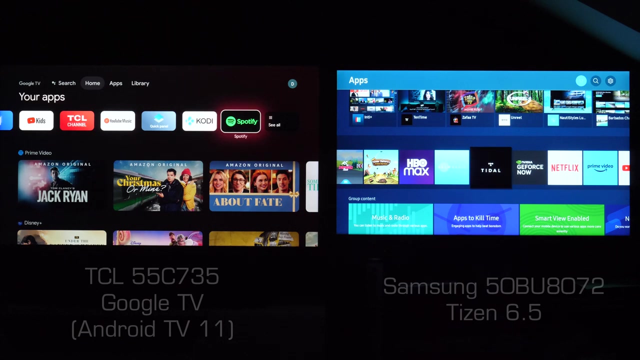 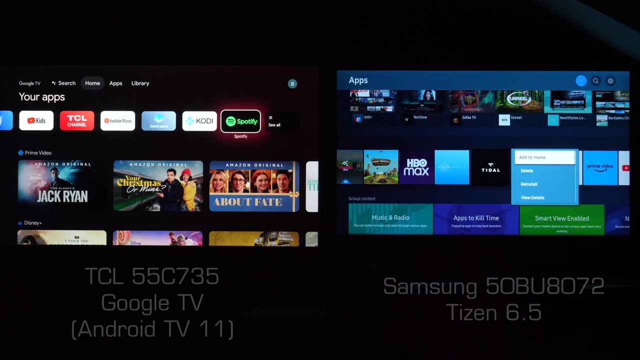 On Tizen. at the end you have this edit list option which just offers move and remove apps. If you want to see all the apps which are installed, you need to open apps menu and scroll to the downloaded app section. Here, for example, if some app is not on the menu then you need to long press, press add to home. 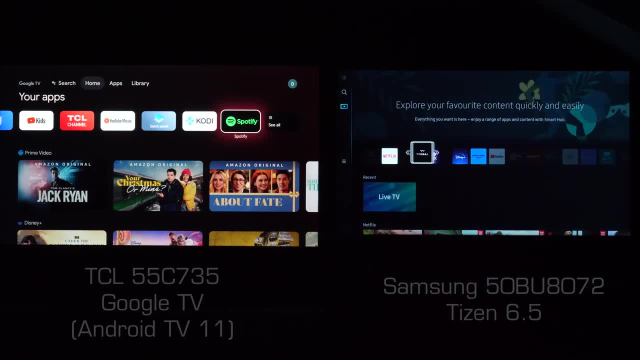 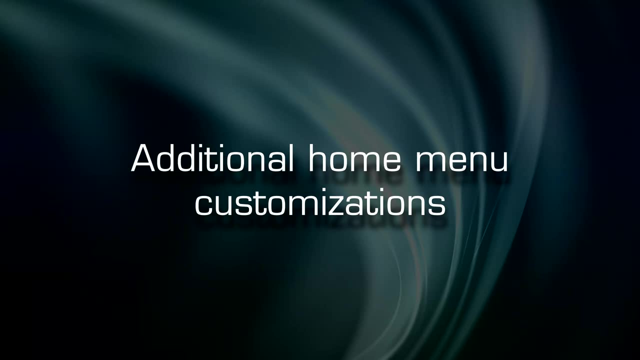 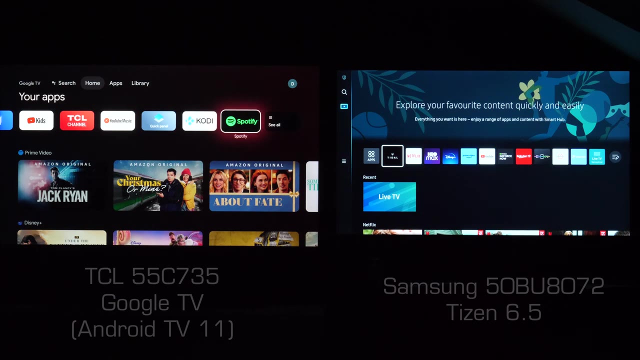 and that app will appear and you can immediately choose at which position to have that specific app. Now, in terms of other customizations, if you want to remove recommended content and so on, You can't do it on Tizen, but you can do it on Google TV. 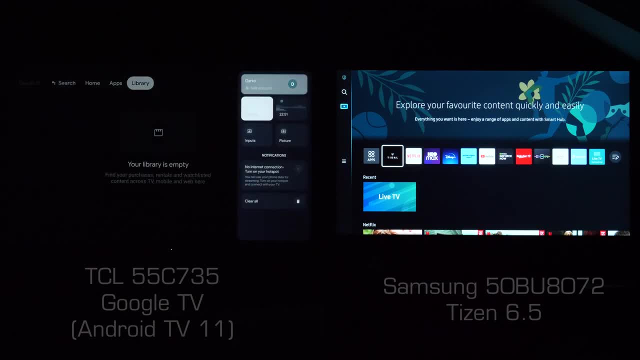 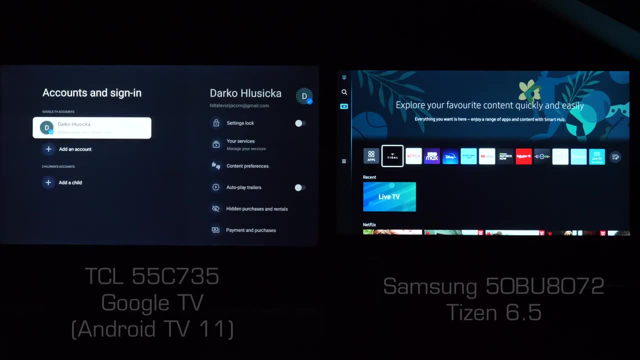 To do it, let's go to the top, to the profile settings, accounts, and sign in. And here, for your account definition, you need to enable apps only mode. So let's go and select accepting custom account content. BoraH, Aquas, baht. 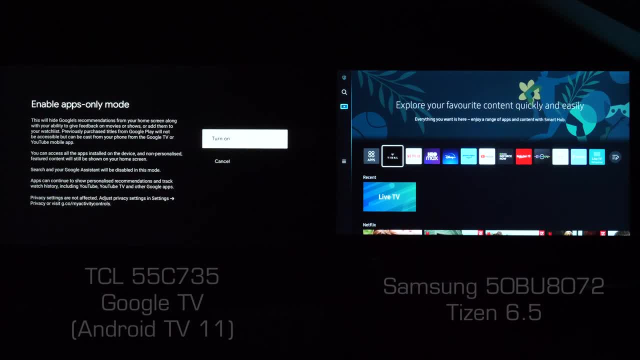 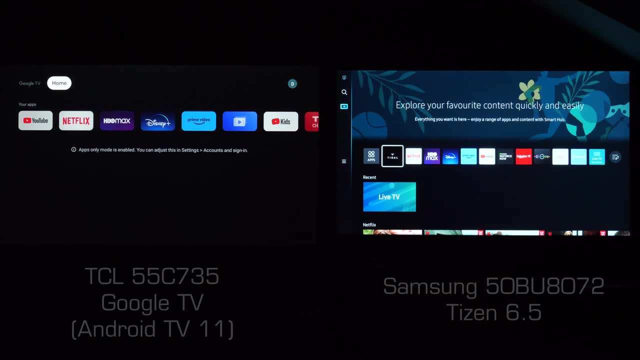 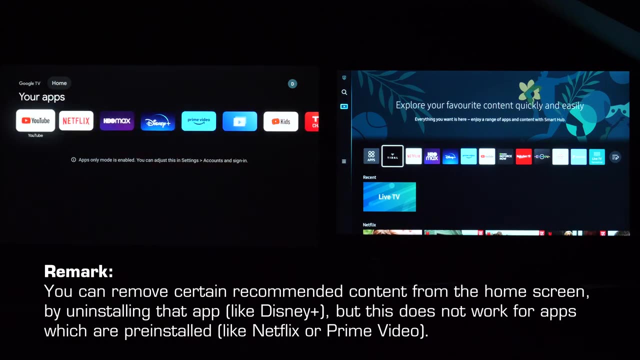 so you will see this notification that this will hide google's recommendations. if we turn it on and go back to the home menu, the home menu will look like this: so you will only see your apps and any other content will not be displayed. so you see simplified interface. 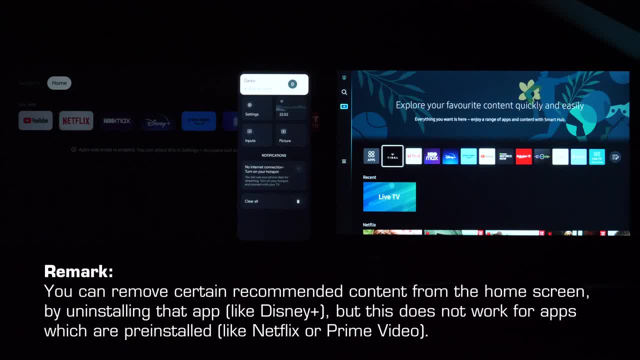 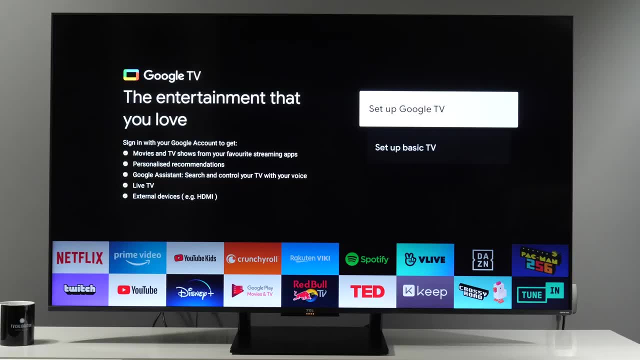 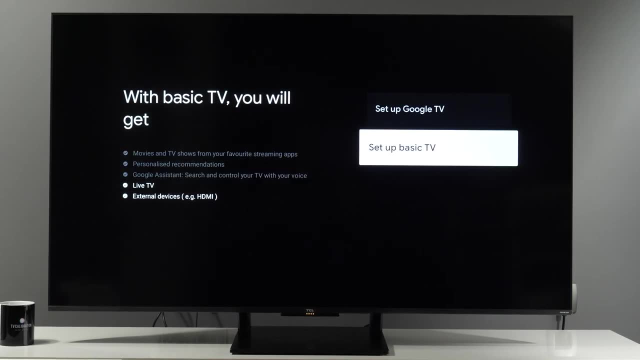 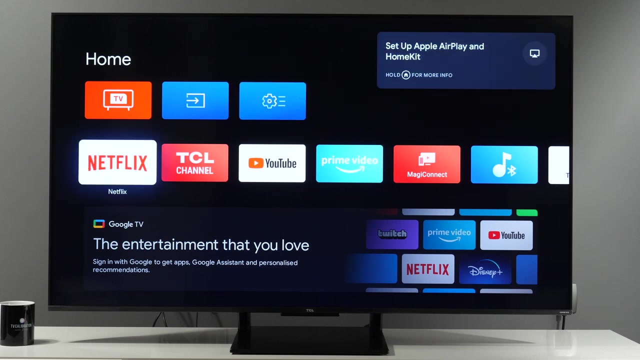 also on top, you only have home and these settings side menu and you can see the default settings for your apps. also, it's worth noting that you can customize google tv interface during initial installation. if you want basic tv functionality, just watch live tv and use pre-installed apps, so you don't need to. 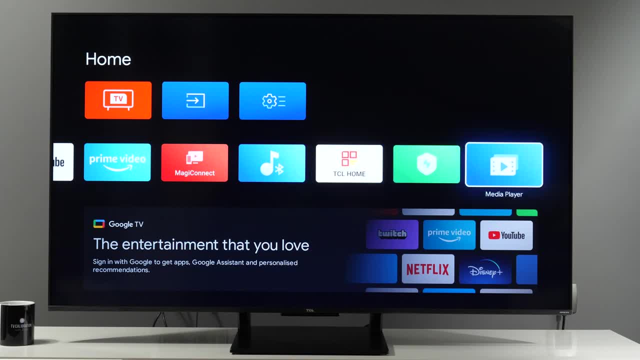 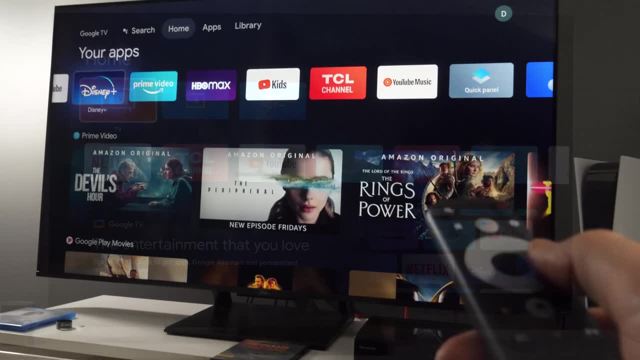 use your google account, then you can use that simplified layout, which is also full screen but it's simpler and easier to use. and if you want all the features, then go with standard function, which is the default settings, and then you can use the default settings for all the features of the app. 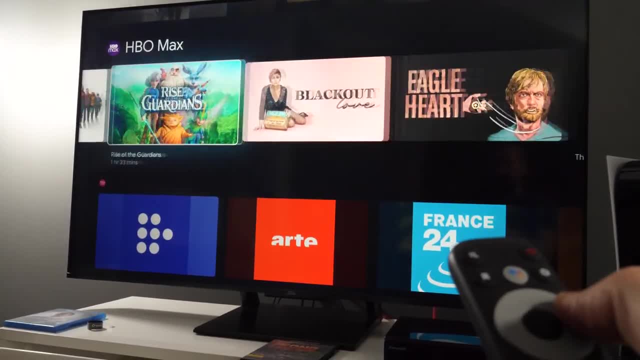 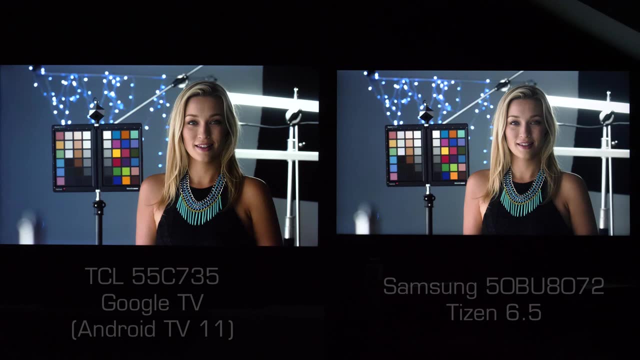 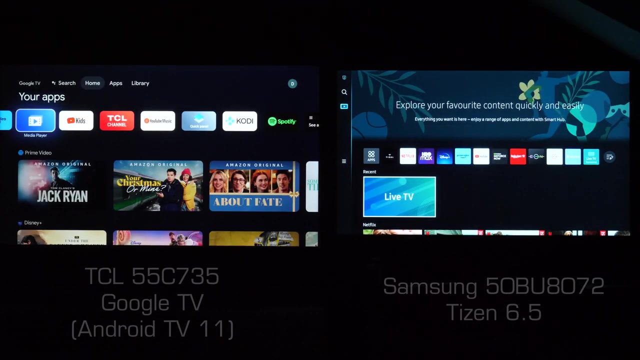 which i'm displaying right now. another thing related to home menu is: can you go back to the content you were watching by pressing back button or pressing home button again? so if i press home button on both tvs, i'm back to the home menu and then, on google tv, pressing back will enable 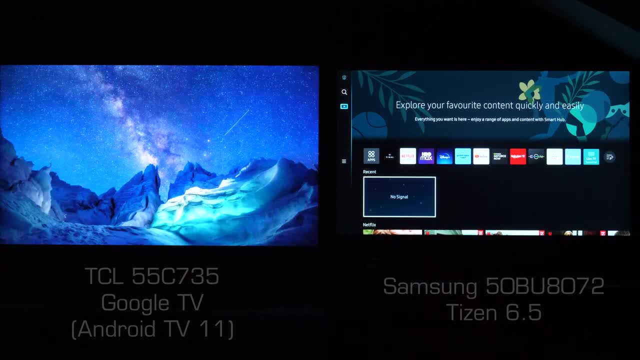 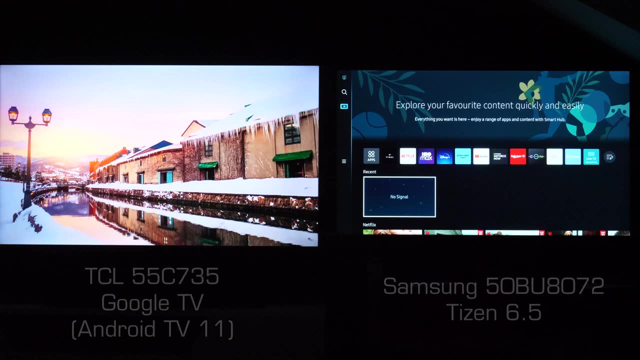 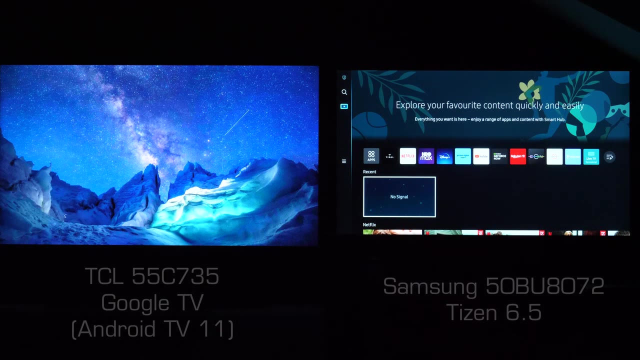 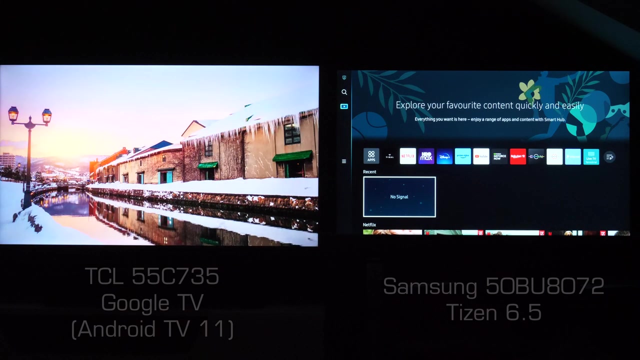 screensaver, it will not bring you back to the content you were watching and on tizen, pressing back will not bring you back to the content that you watched before. what i did was i was playing a static content from my local server on both tvs. so to come back to that content, i will open media player on. 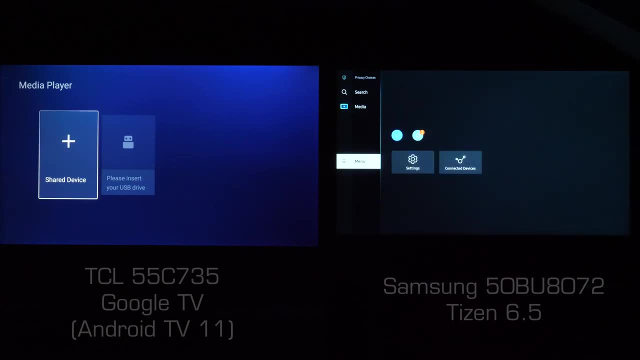 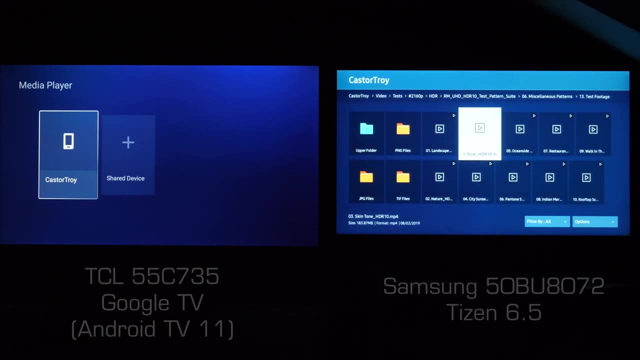 google tv- and here i will go to menu connected devices- caster troy and i'm immediately back to where i was while on google tv. i need to go back all the way through the folders to find that same content- test footage. so we are right here. skin tone. 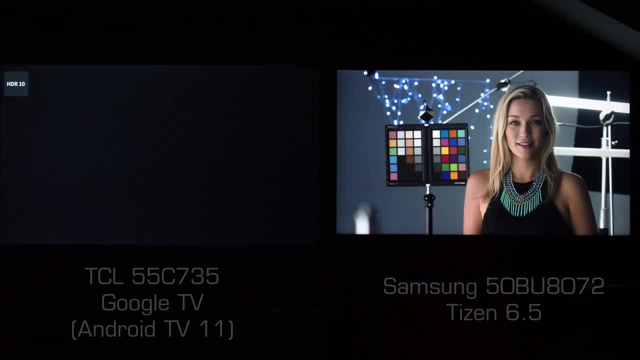 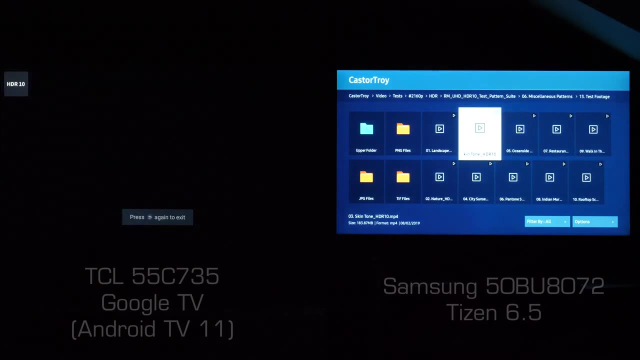 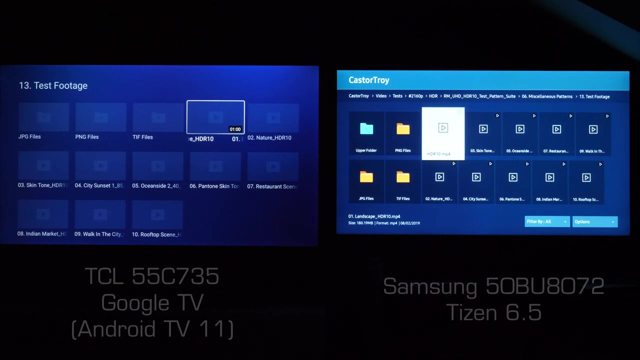 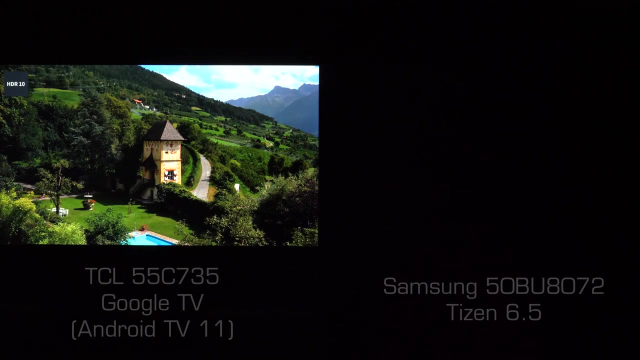 i'll press ok at the same time. and here we are. and then let's go back on both tvs and open some other content. let's go with landscape three, two, one. okay, we see it on google tv and tizen is still loading the content, but again. 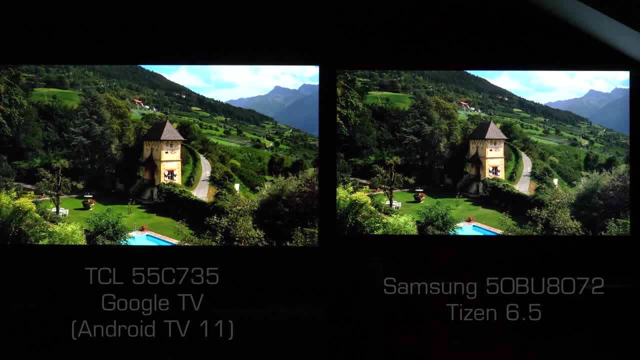 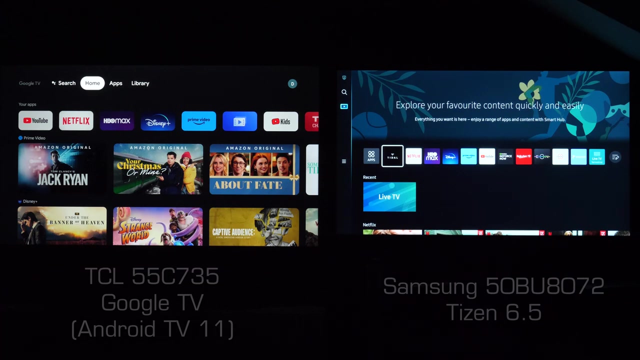 consider that, uh, this is not samsung's ql voice line, this is 4k uhd line. so more expensive tv will have faster processor and tizen platform, which will work faster and tizen platform will be faster. both tvs are offering different profiles. mainly that you'll log in with your own account and have 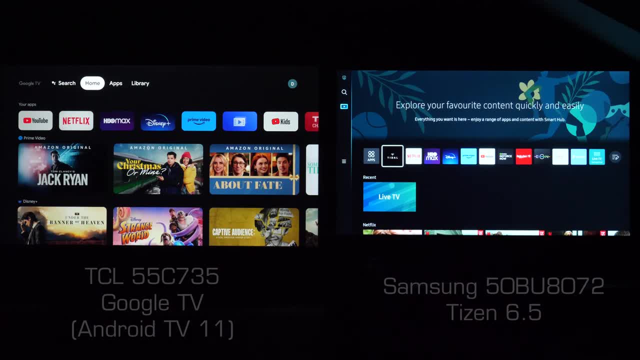 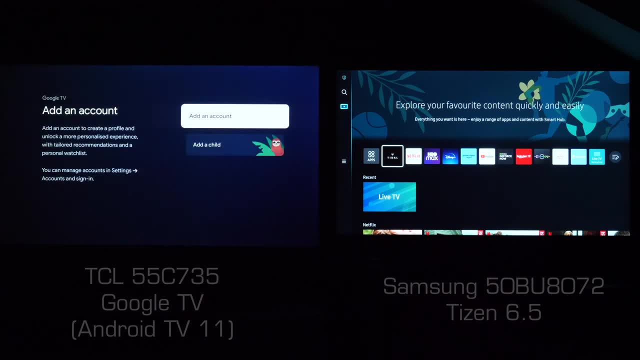 your own recommended devices and connection to facebook and other different services as well. the viewing of themselves will also beены devizers displayed On Google TV. you need to go to the right click on add account and here you can add it, and you can add your Google account or add a child On Tizen. 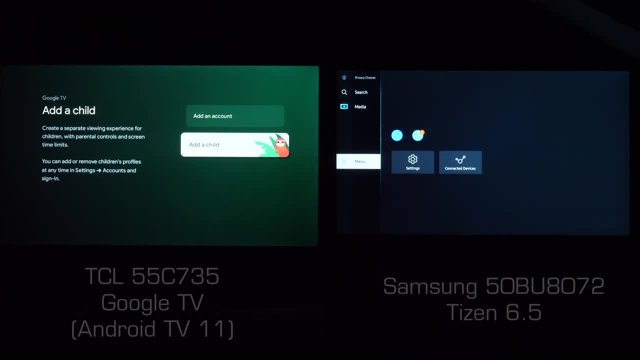 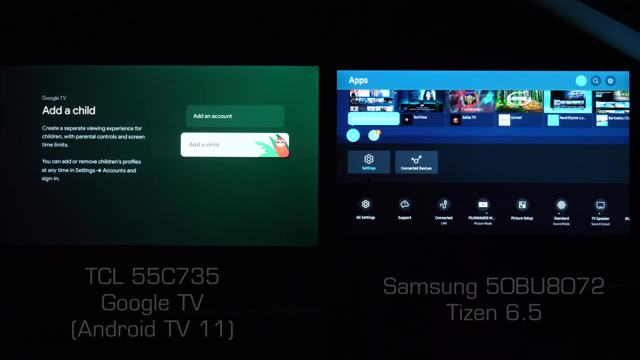 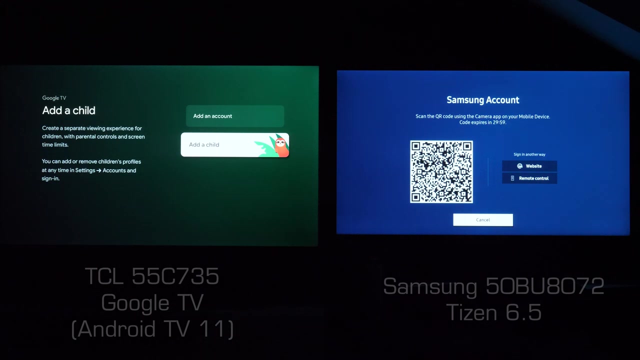 what you need to do is go to the left, to the menu, then to the right, then to the top, click on your current account, and here you can sign in with another count that you have or you can create a new one, the option which is also. 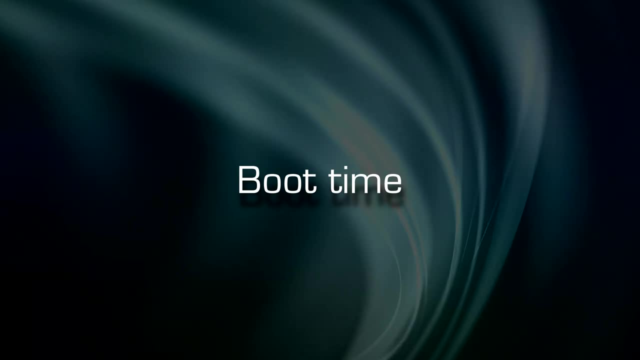 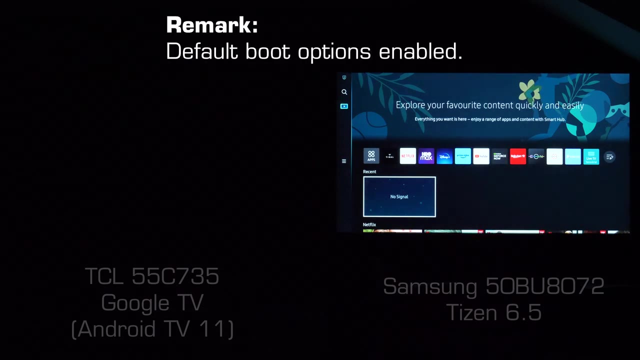 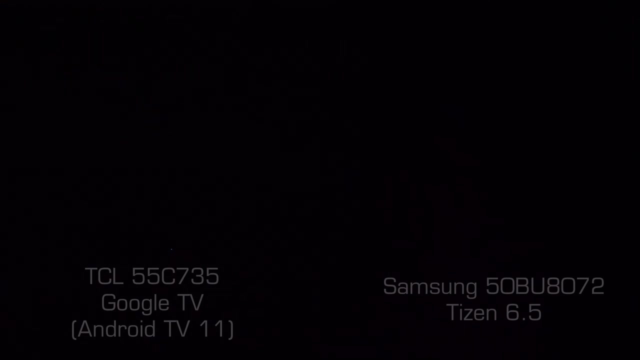 available Now. I'll show you how long does it take for both TVs to come out of standby, so I turned them off now. let's wait a few moments until they are turned off, and now let me see if I'll be able to turn them on at the same time. yes, so as you. 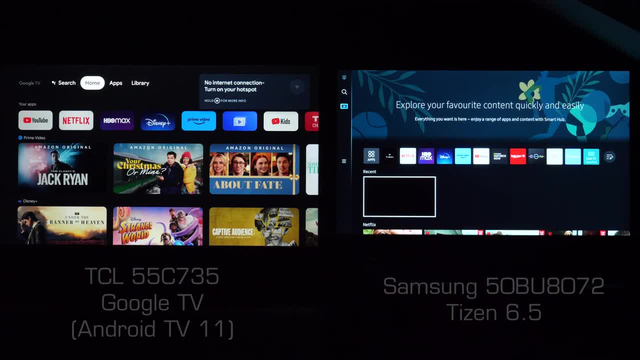 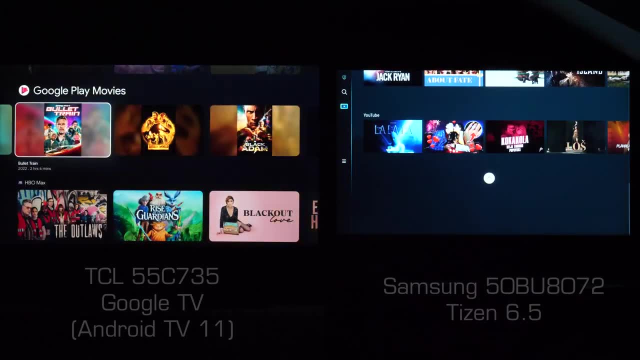 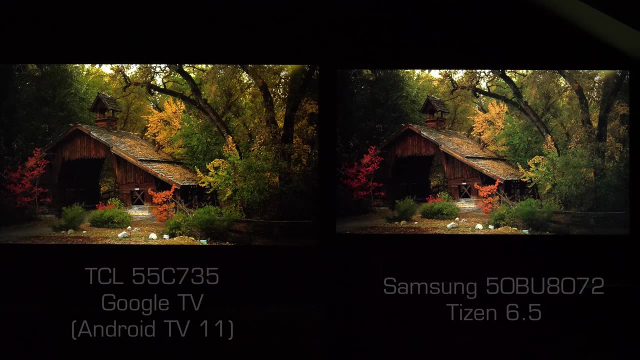 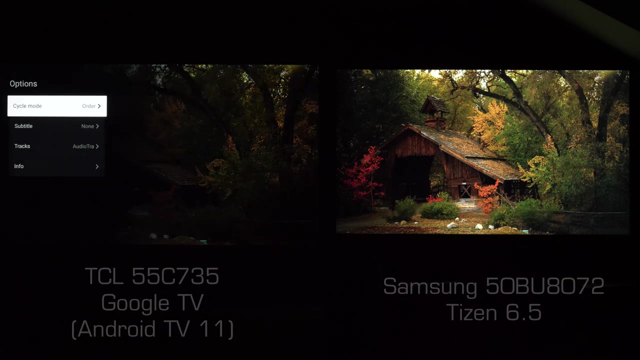 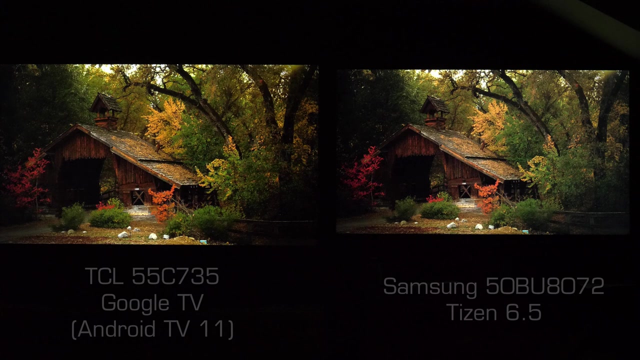 can see. within a couple of seconds you see home screen and you can move. you see everything is reacting fast in terms of different side menus which you can open during playback. on Google TV, you have this settings menu where you can see info about playback, and there is 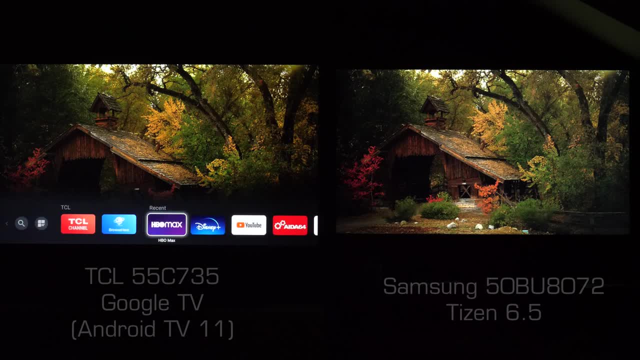 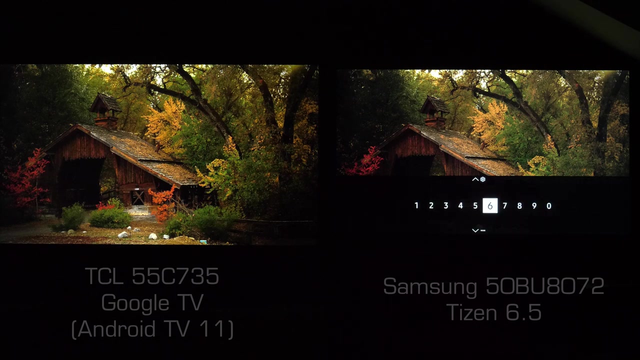 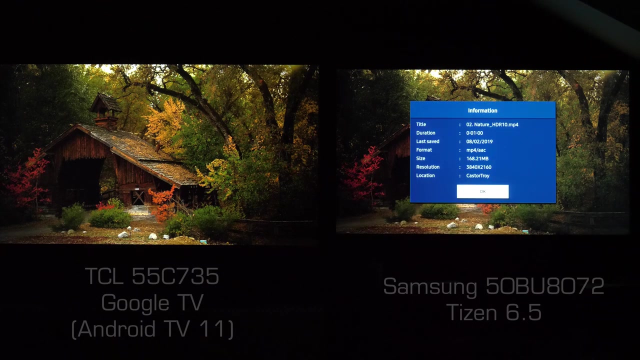 also this bottom menu with recently opened apps: TCL content, TCL channel and web browser, TCL home search, multi-visual input settings and so on, and on Tizen, if you press settings button, you will also see menu appearing below with numbers, with settings, and the third line is info, so you also can see information about the content. 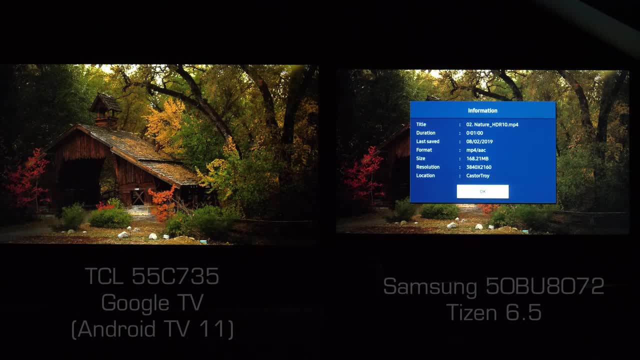 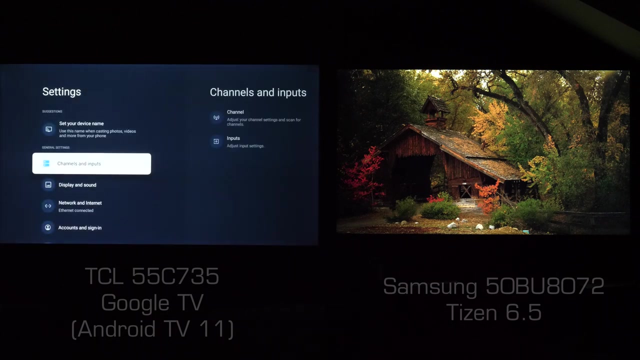 specifically, I'm in built-in media so you can see information about the content. specifically, I'm in built-in media player right now, so I see this content. of course, different inputs will show different information in this regard. in terms of the settings menu on Google TV, you press settings button to open this full menu on Samsung. let's go to all. 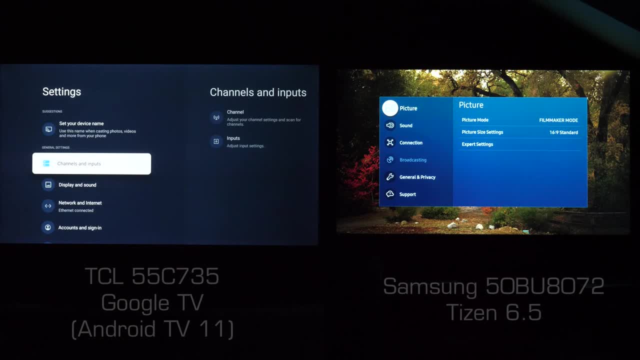 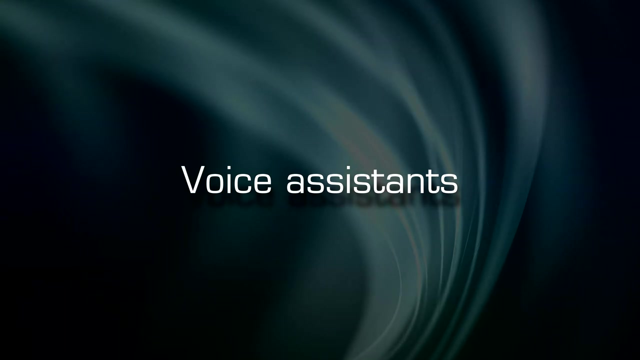 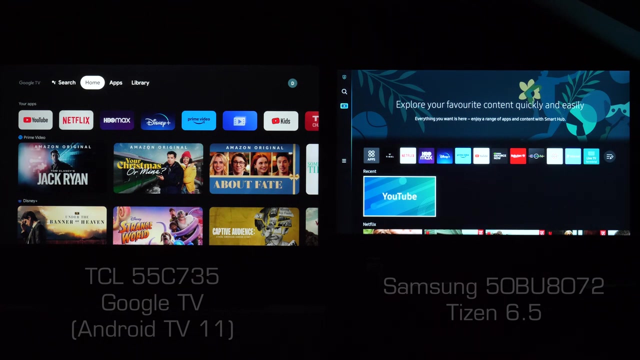 settings and you see menu appearing at the center of the screen. Google TV has different options: set your device name, channels and inputs, display and sound and so on- and Samsung has picture, sound connection, broadcasting general and privacy and support. both platforms offer voice assistance so you can open different apps and settings. 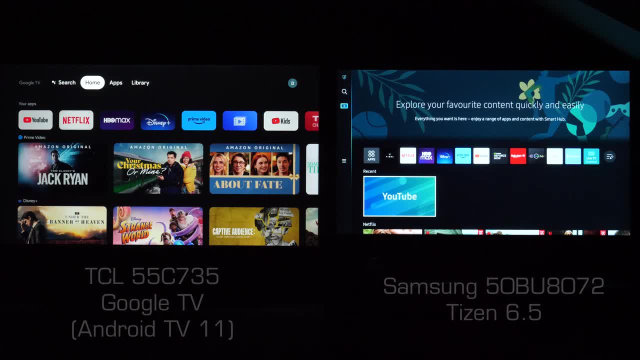 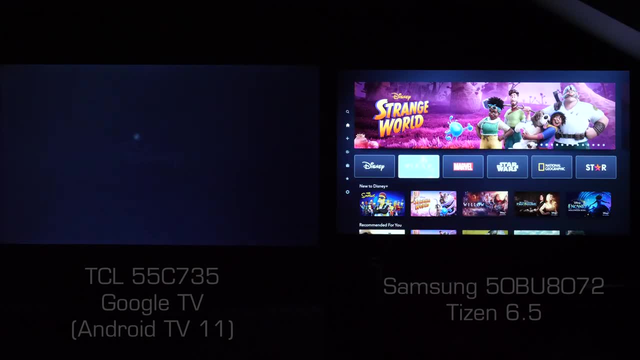 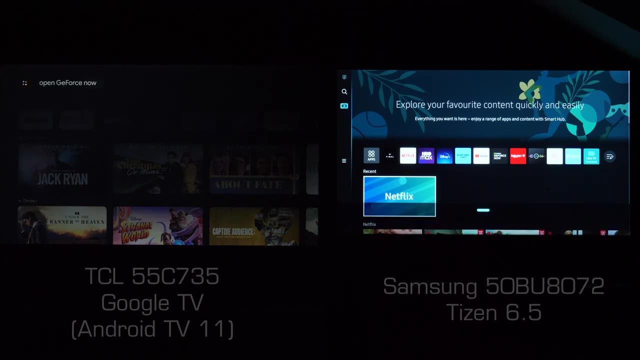 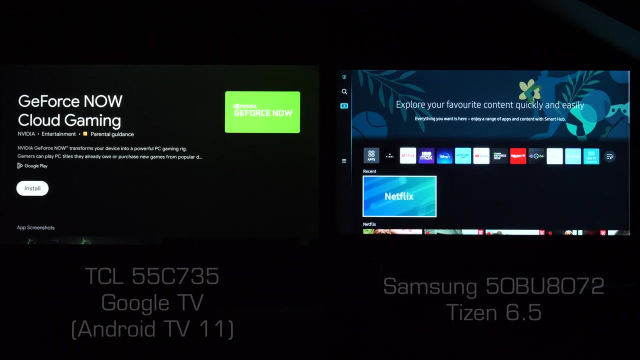 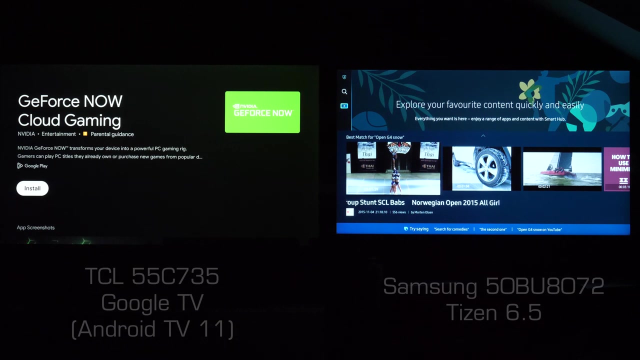 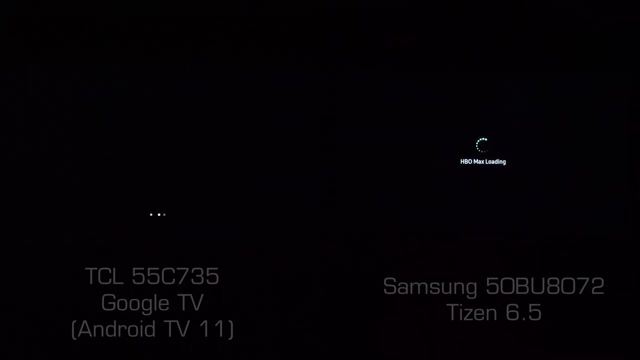 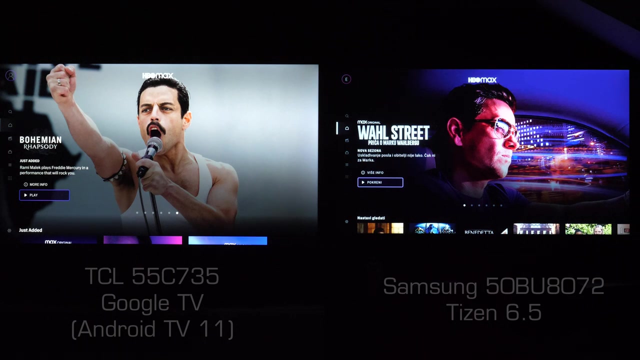 let's see how it works. open Disney Plus. open GeForce now. open GeForce now. so you see, Tizen is not opening the app and Google TV is offering to install that particular app. Open HBO Max. so definitely, you can use voice assistants to open apps easily, especially on models which have built-in microphone in the TV itself. so 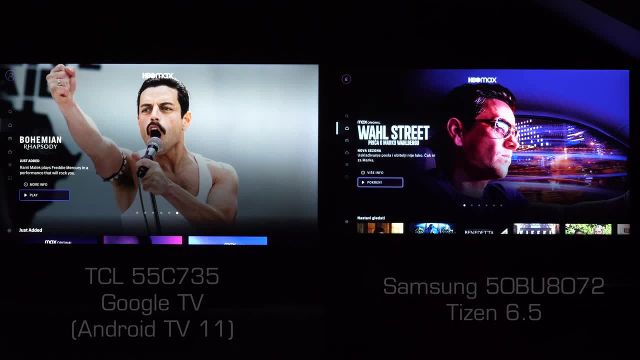 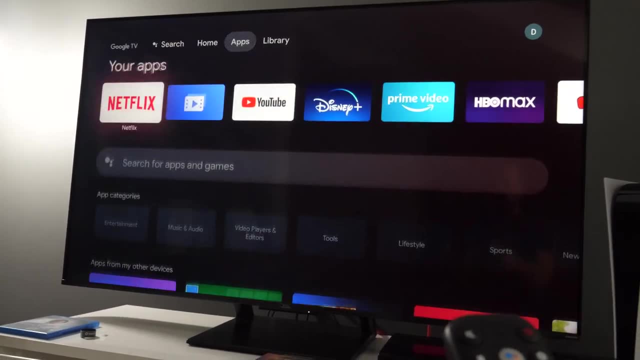 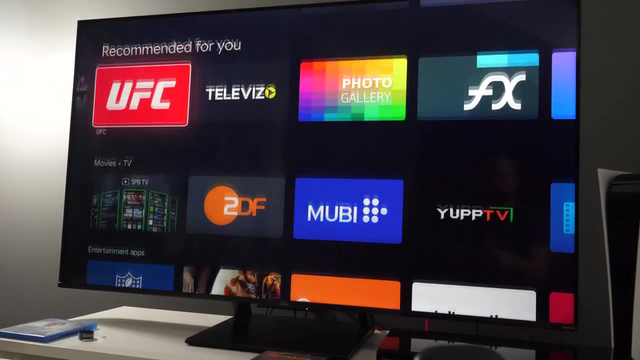 you don't need to use the remote control. In terms of stability, both platforms perform well. all the streaming services are playing content smoothly and without skipping frames. What I did notice on Tizen OS are occasional slowdowns in the audio quality, So you don't have to worry about that. 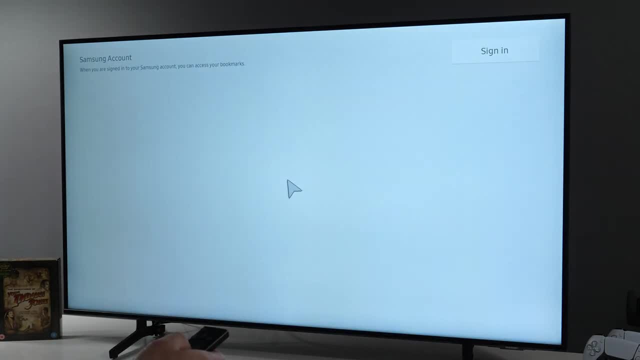 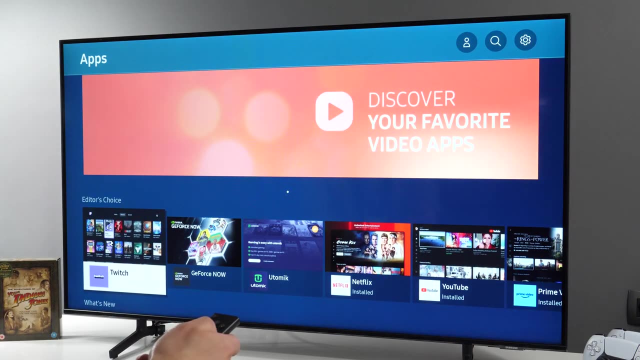 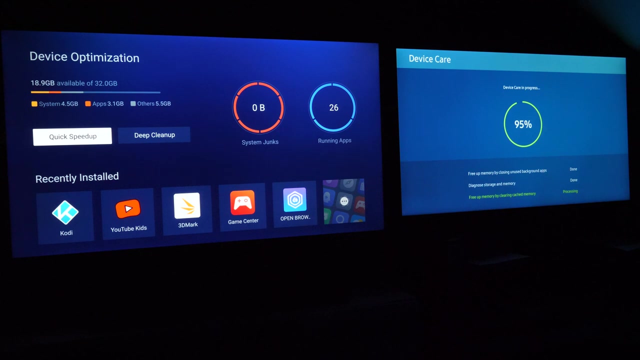 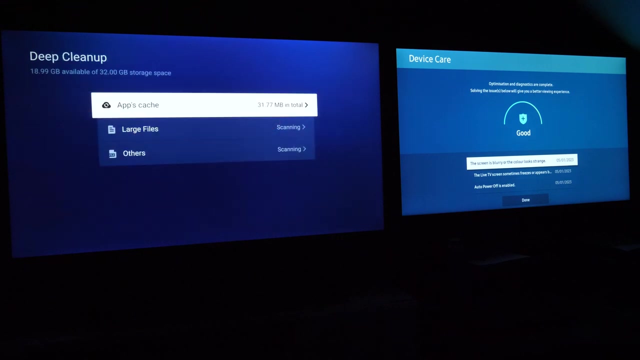 Inside the menu. as I was scrolling through different options, sometimes the screen would stop, and this was happening on both this specific TV as well as Neo QLED QN90B that I tested before. If you notice stability issues, both platforms offer services for system optimization. you can look for them inside the menu. 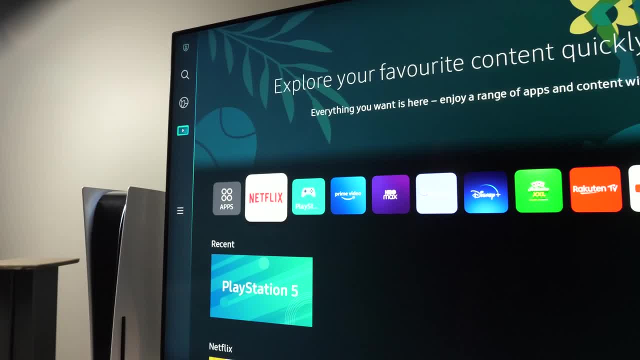 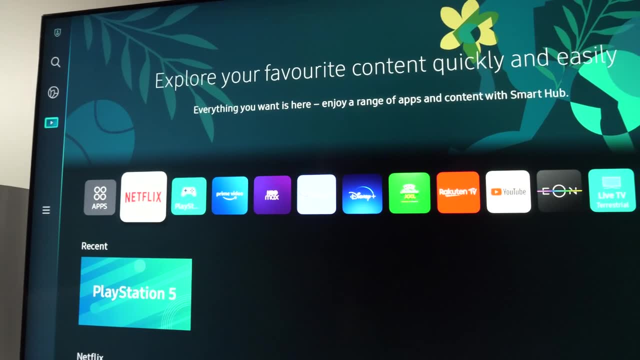 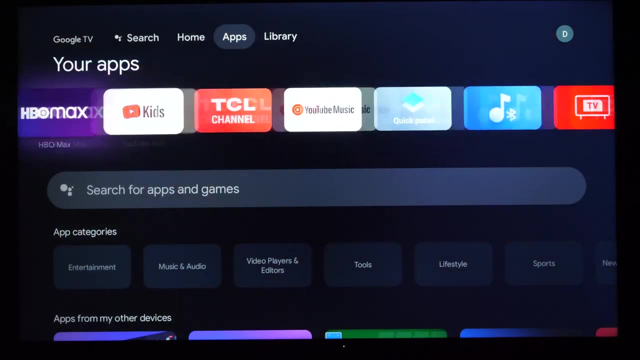 And with this, ladies and gentlemen, we've come to the end of this video. I hope you got a feeling of what both platforms offer. Google TV has an advantage in terms of number of apps available inside the App Store, While Tizen is more limited. 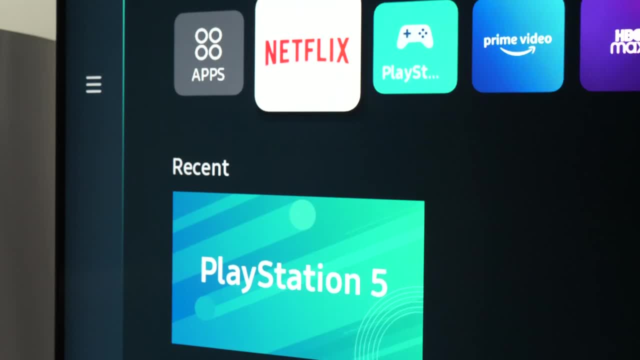 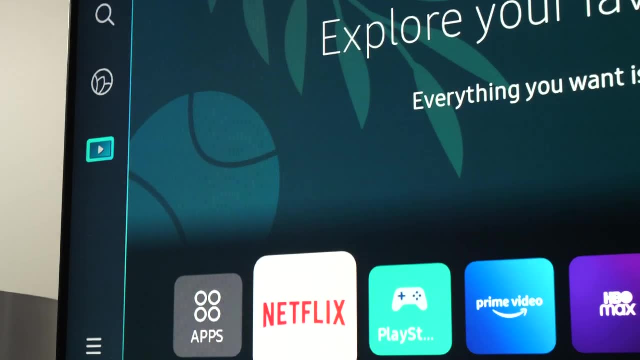 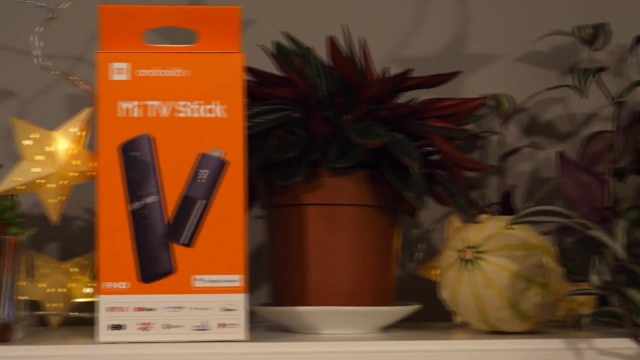 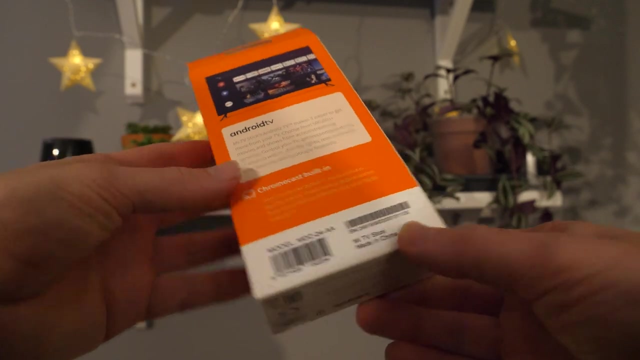 and even though we will find all the popular streaming services, if you want specific apps for streaming, like Kodi and so on, Those apps are not available and the only solution to get them is to buy Android TV stick or set-top box and connect it via HDMI port, and then you will have also Android TV.